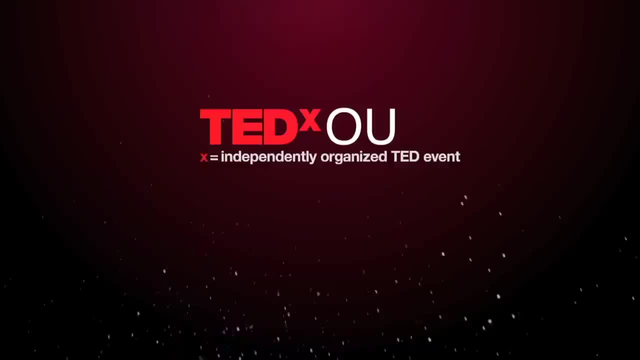 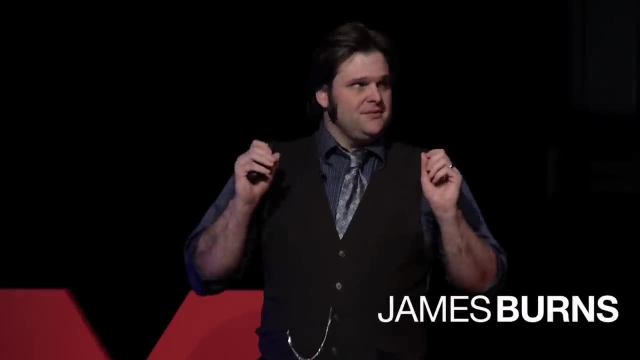 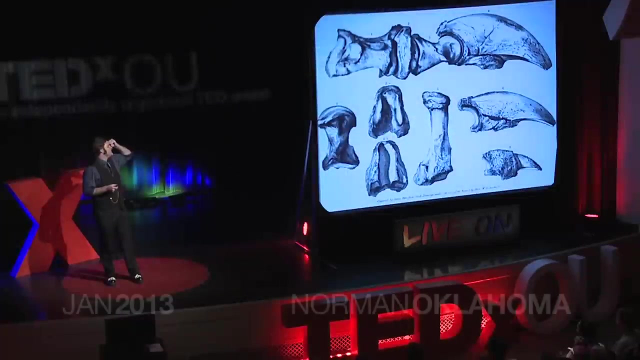 Don't discredit something or ignore it just because it seems familiar. Now, this probably doesn't seem familiar, but we'll get there. In 1796, Thomas Jefferson was in an argument with a count in France about the degeneracy of the United States. The US was in the new world. It. 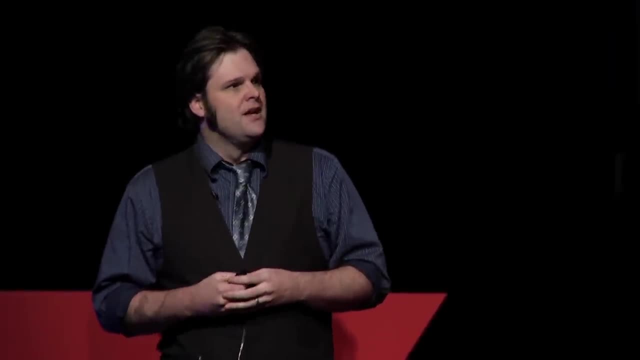 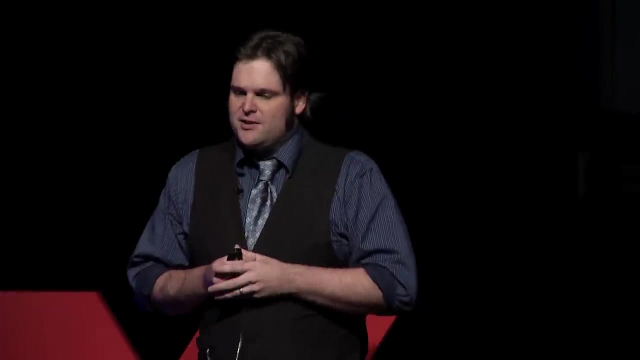 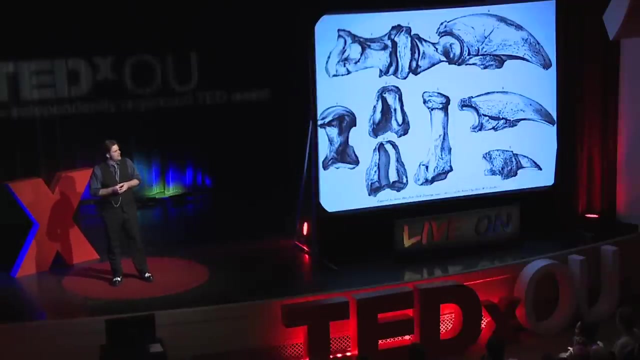 didn't have anything as big and as gallant as the old world, And Jefferson, being the man that he was, was absolutely sure this was not true. These bones arrived on his desk when he was vice president. He looked at them- The largest claw there is seven inches along the curve- And he 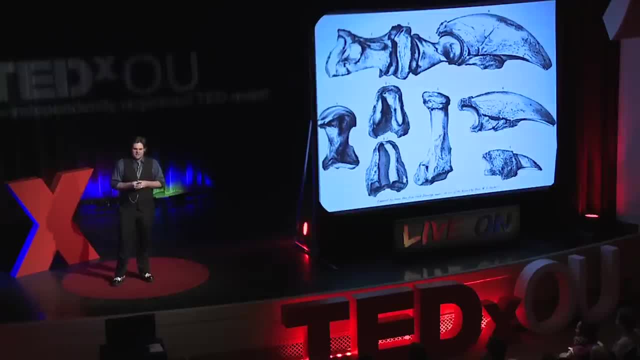 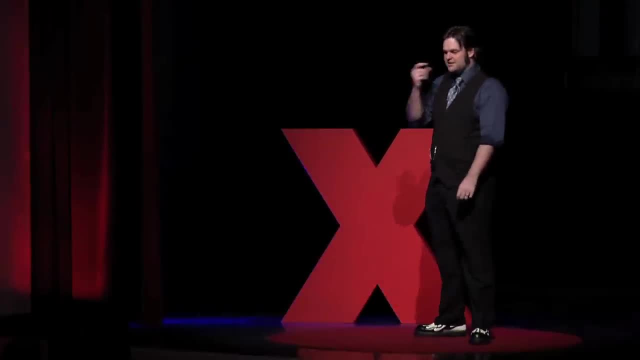 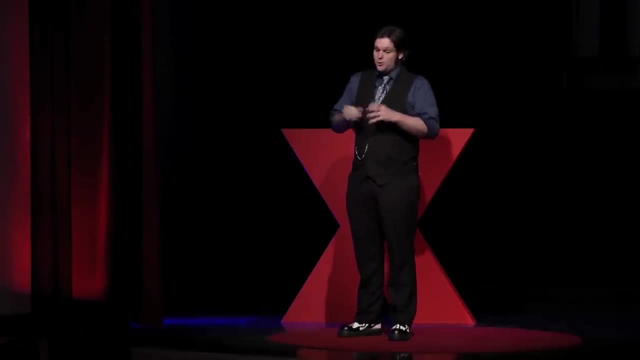 says: hmm, this is obviously an American giant French count eating lion, And he described it. at the American Philosophical Society in Philadelphia, The vice president sitting vice president gave a scientific paper on fossils, proving that America was not degenerate. However, it was later proven that these were actually a. 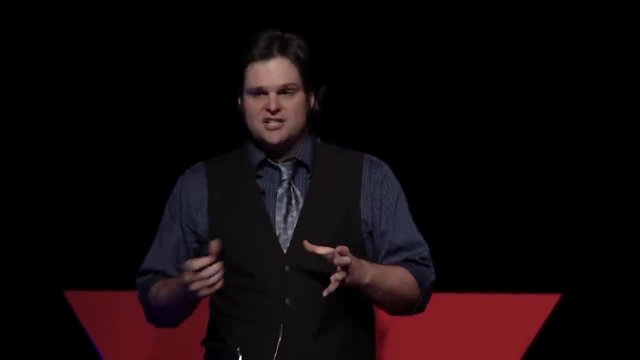 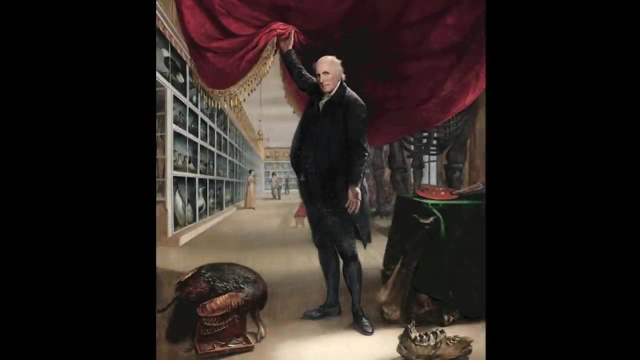 giant ground sloth and not a lion. Still a giant, not vicious. Here's Charles Wilson Peale in 1801 in his museum. He led one of the first scientific expeditions to the United States. He was a scientist in the United States to exhume a monster. You can see it peeking out from under the 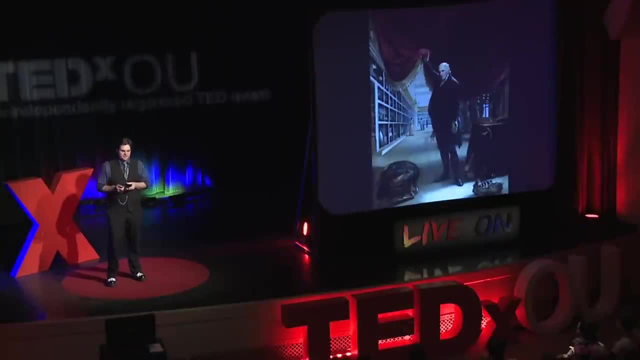 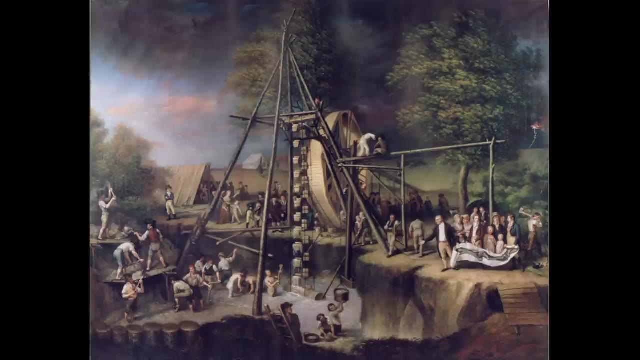 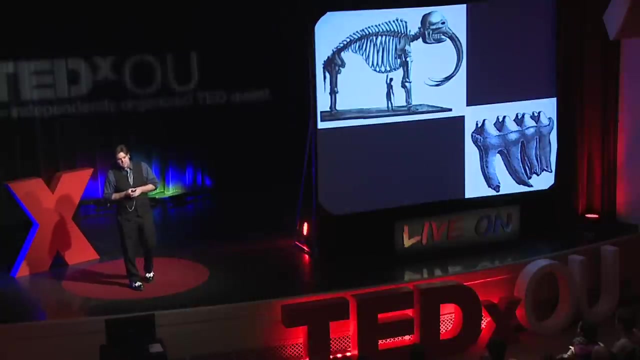 curtain And his tooth is there on the bottom right. He designed the machinery. His entire family helped exhume this mastodon. It's in upstate New York. They put it together based on the pointy teeth. It obviously eats meat, So therefore it was a saber tooth. mammoth Sneezing was probably the 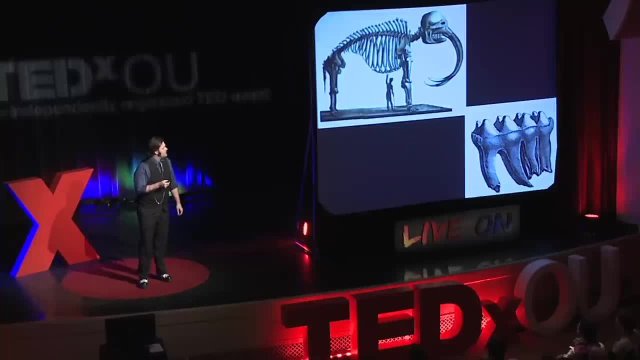 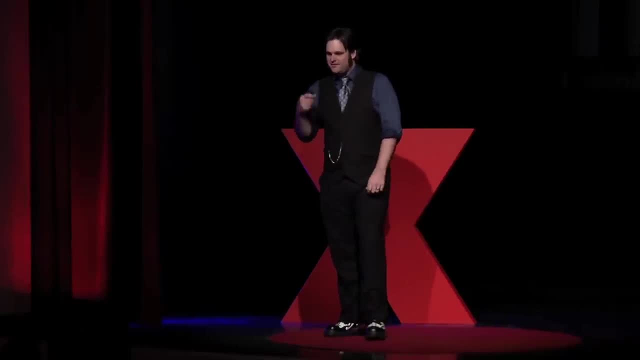 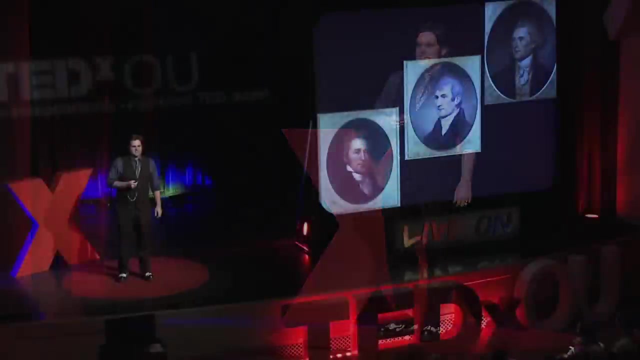 cause of the extinction of this creature. However, after touring in Europe for a while- very short while- they actually flipped him around and realized this was a mastodon, Thomas Jefferson is now president. He hires two men to go on a long walk. These three paintings are actually.